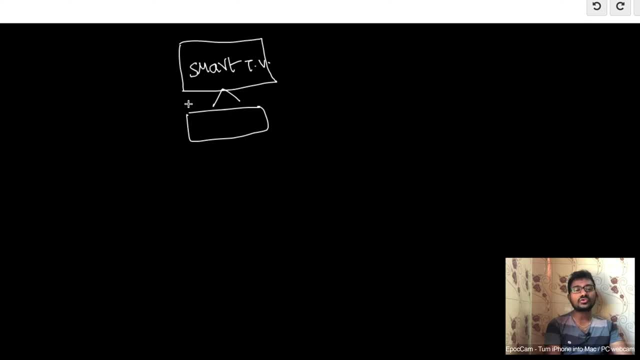 So they are trying to sell the most demanded product. So Flash Sale means the Flash Sale will last only for 2 to 3 seconds, So if you are lucky, you could buy this product at that time. So the Flash Sale would be held on every week or on every monthly or weekly basis. 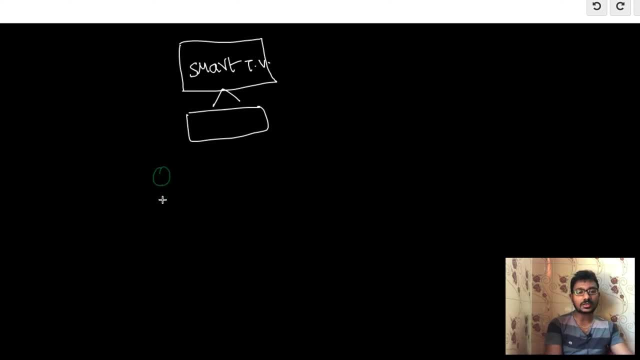 Suppose if 4 people are willing to buy this product, So this is the second one, third and fourth one. These 4 people are trying to buy this product, But for the first time they have failed to buy this product because of stock unavailability. 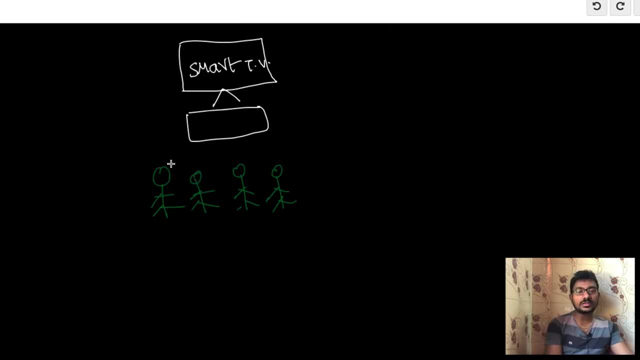 So what they are trying to do is they are trying to register with this product on that online site. So whenever this product is available, then the notification would be sent to these people. So this subject will send the notification to the registered people. 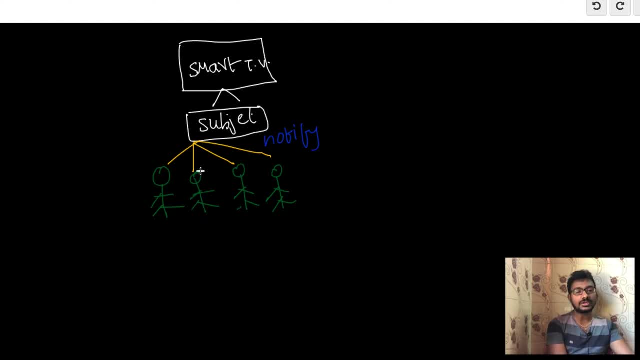 So here we can relate the Smart TV as a subject and these people as observers. So these people are observing something, These people are trying to buy the product, So they have registered with this subject. Whenever the product is available, the notification will be sent to these observers. 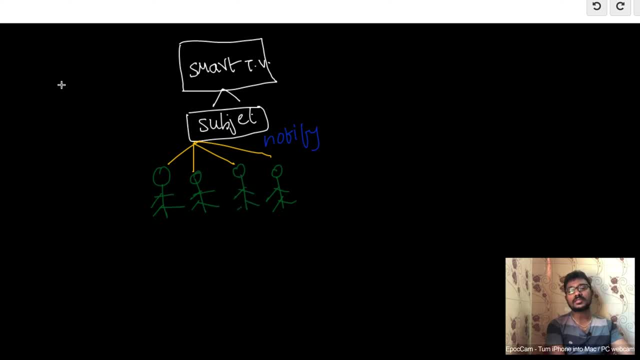 So these are the observers. We are trying to buy some product and we are trying to register with them. So here: first observer. second observer, third observer, fourth observer. The first observer doesn't know the information about the second observer. Second observer doesn't know the information about the third observer. 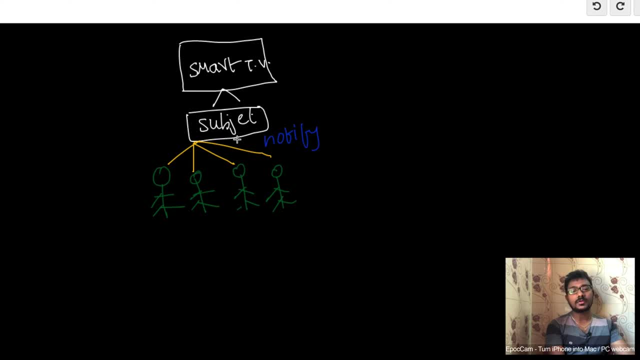 But all the information would be available for the subject. So A, B, C, D. So these A, B, C, D are the observers. Subject: would hold the observer IDs, Which means A ID, B ID, C ID, D ID. 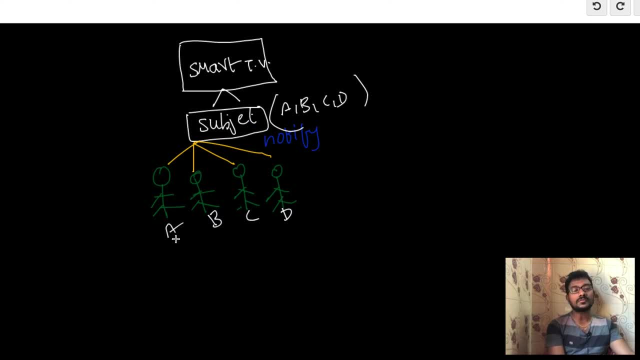 Subject won't hold all the information about all the observers. Subject won't hold the observer name, observer details, observer city observer, previous purchase, etc. Subject would hold only the observer IDs. So this is the example where observer design pattern is playing a major role in real life scenarios. 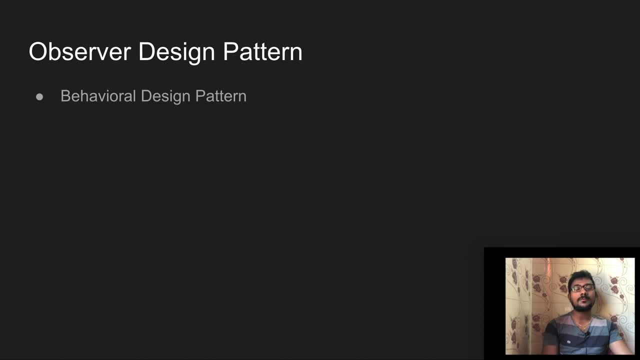 We will try to relate these points with this example. So first one is behavioral design pattern, Behavioral design pattern. This observer design pattern falls under behavioral design pattern. The reason behind that is it behaves based on some state. And then second point is object or subject maintains all its dependence, called observers. 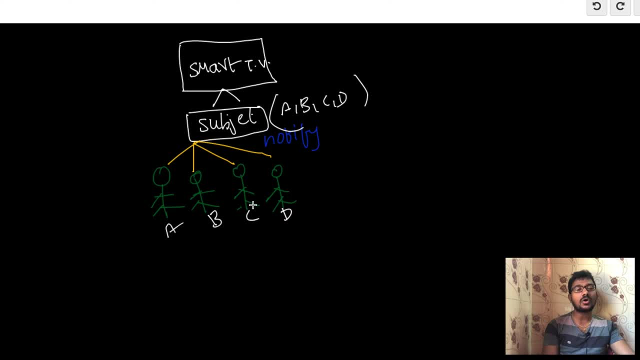 So here this is a subject or object which maintains all the information about the, all the, not all the information- which holds information about all the observers. Here it holds only the information about the observers as observer IDs. So it holds the observer A ID, observer B ID, observer C ID and observer D ID. 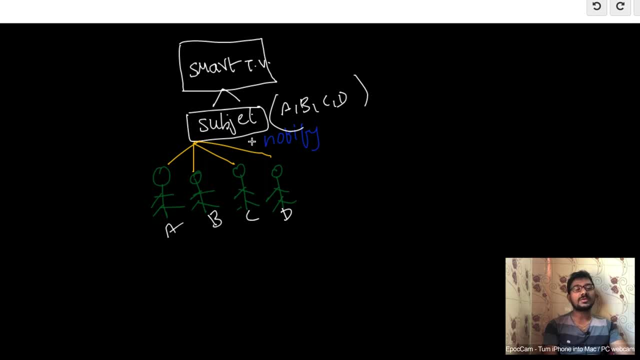 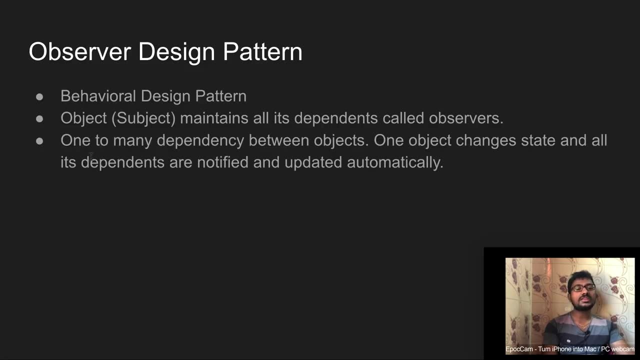 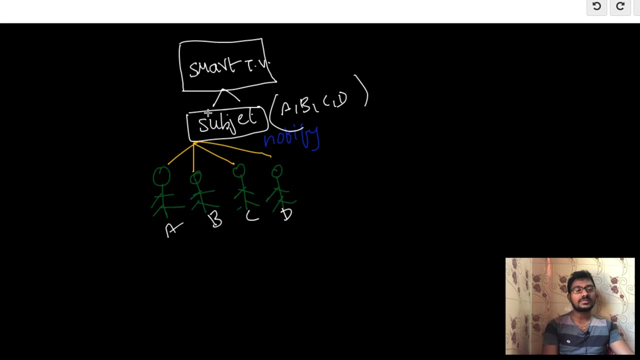 It won't hold the observer, A personal information like name and the other stuff. It holds just the ID for communication And then one to many dependency between objects. One object changes state and all its dependence are notified and updated automatically. So this is the subject. 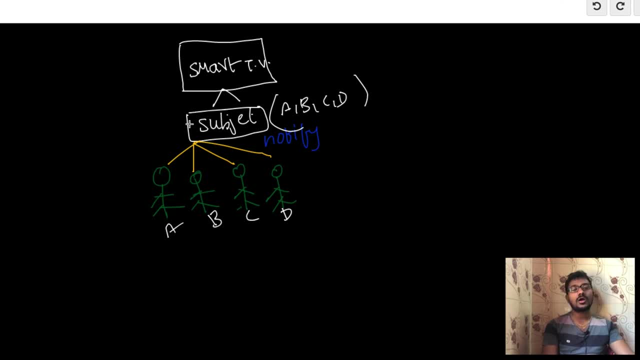 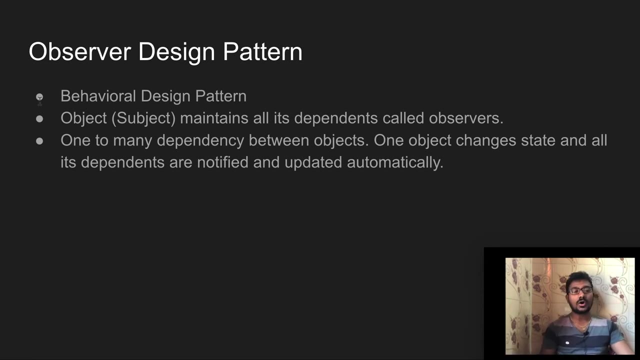 If suppose this subject is changed from unavailability to availability state, Then all the observers, which means all the objects which are registered to this subject, would be notified. That is this point, One to many: dependency between objects. One object changes state and all this dependence notified and updated automatically. 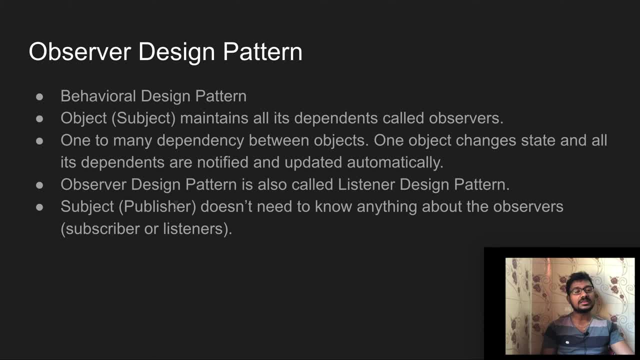 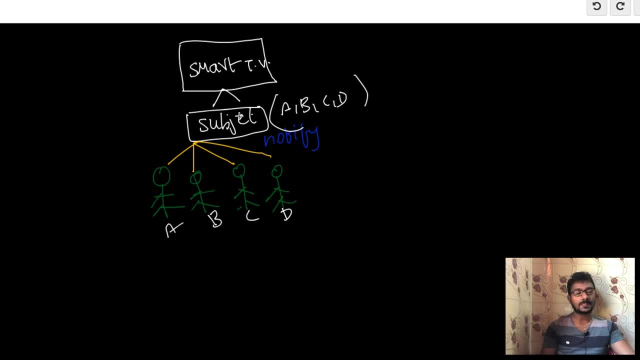 And another point is: subject or publisher doesn't need to know anything about observers or listeners. So I've already talked about that point in the while explaining the example. Subject doesn't maintain all the information about all the observers, Like it won't maintain the observer A personal data like name, age, date of birth and other stuff. 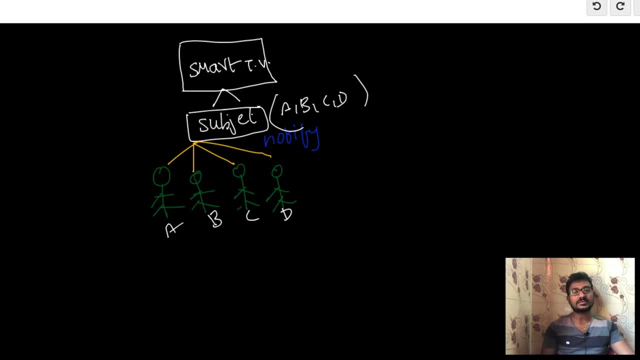 Subject would hold only the observer. A ID, That's it. And then very loose coupling. Here A, B, C, D are observers, They are linked with the subject. So here one to many, dependency, Subject one and observers are many.